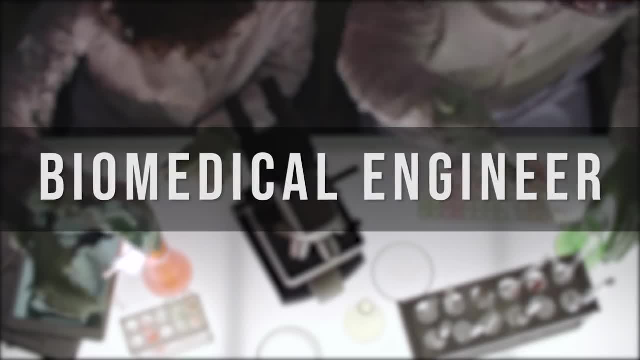 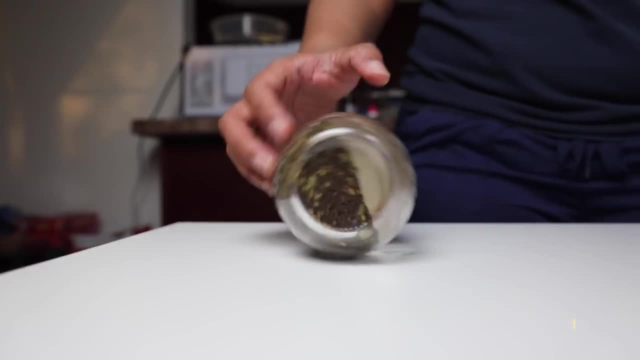 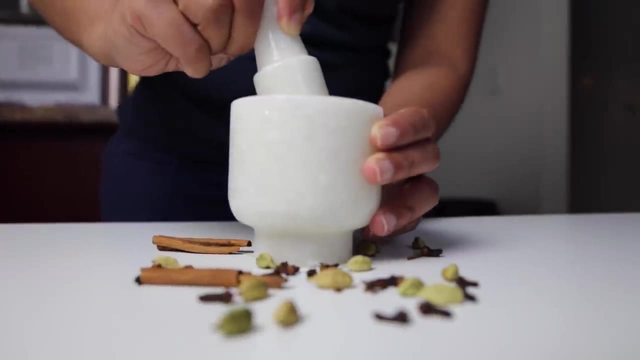 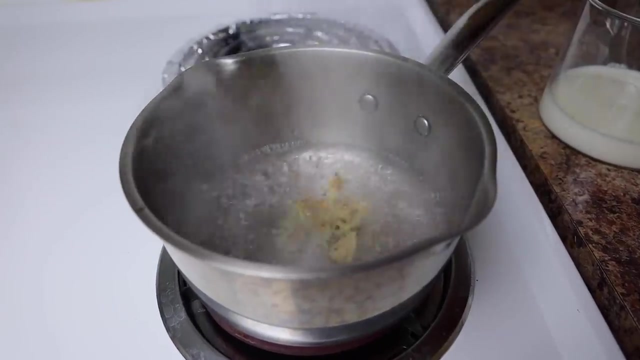 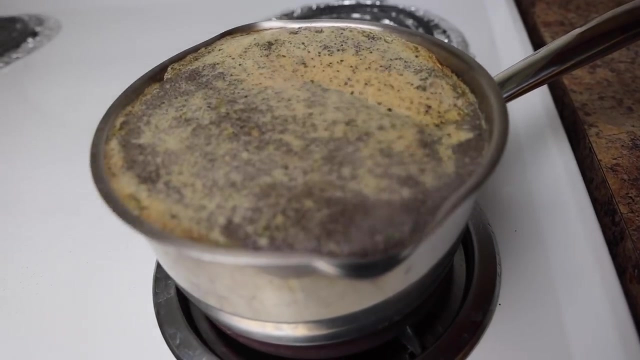 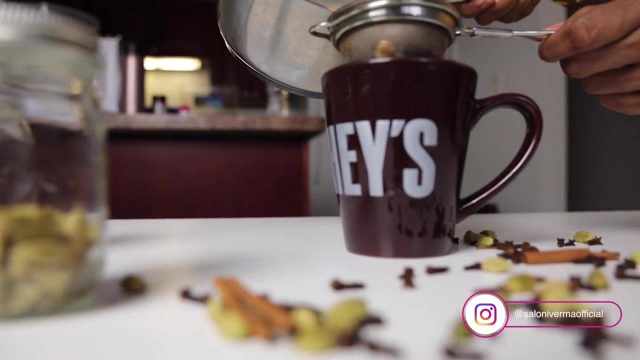 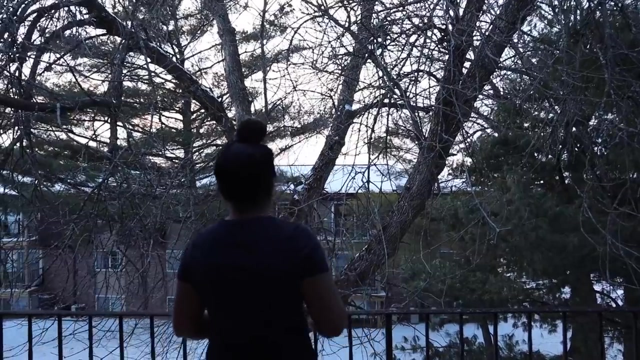 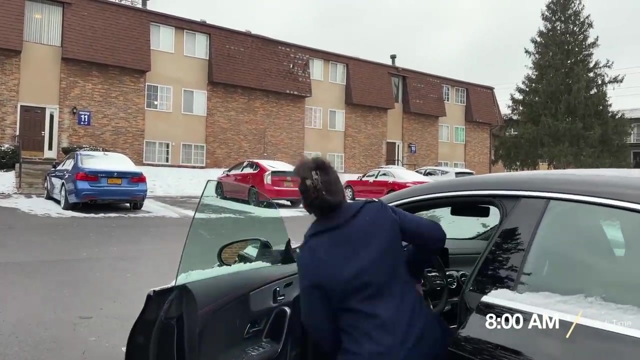 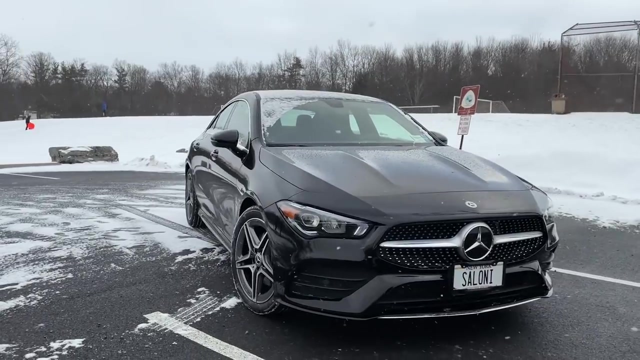 Hey Bill, I'm in the mood for a switch up. I hit the function, hit the rosé till I hiccup. I'm in the mood for a switch up. I hit the rosé till I hiccup. What's going on, guys? Welcome back to a brand new video. and there are just so many of you today. 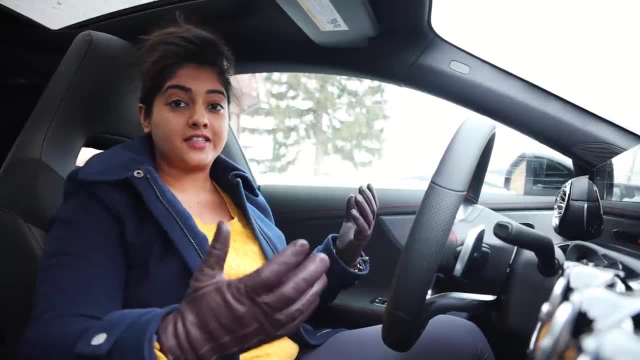 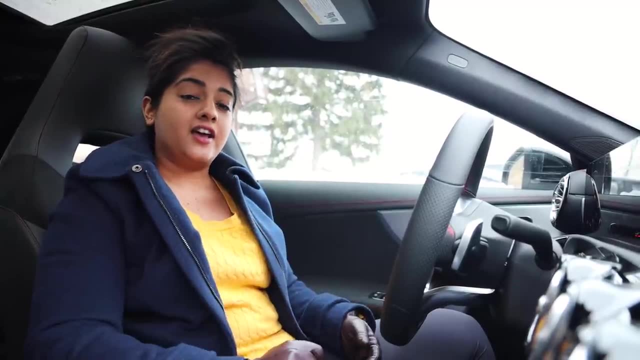 So, without any further delays, let's get started with this day in the life video. For all of those new people who are new to the channel, who don't know me, my name is Saloni and I am a biomedical engineer. I live in New York and, as you can tell from the 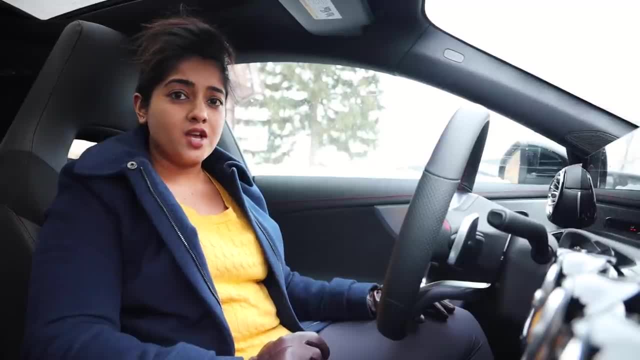 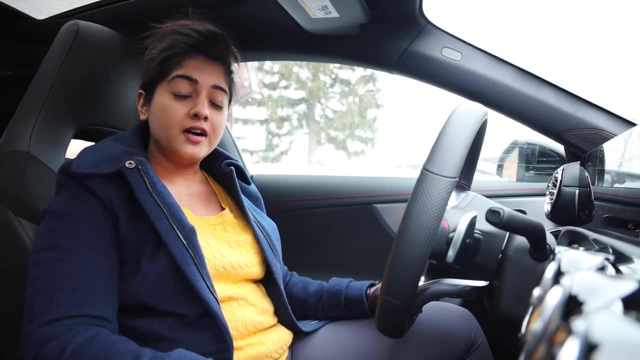 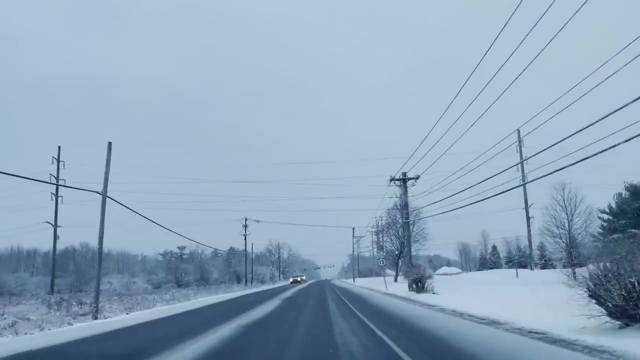 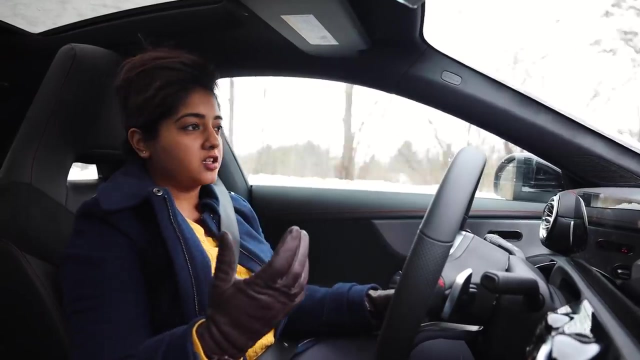 weather. it's snowing. It's minus seven degrees Celsius today, So it's a cold morning. I barely got out of bed, but we're going to head to work now. I'm going to take you guys along. So, as a biomedical engineer- if you guys haven't watched my previous video, I talk about what a 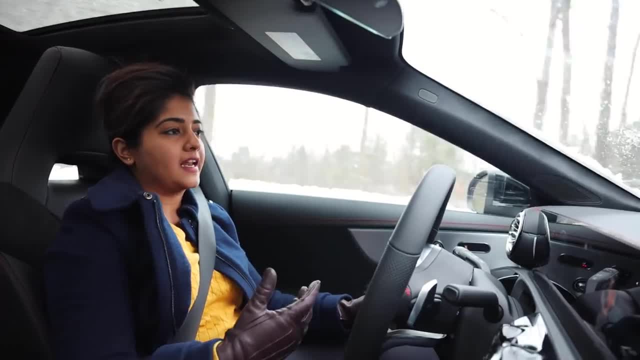 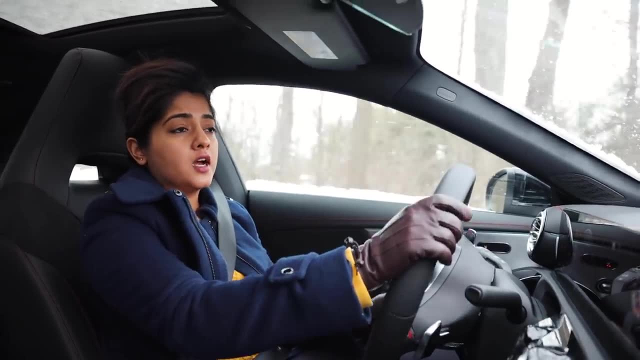 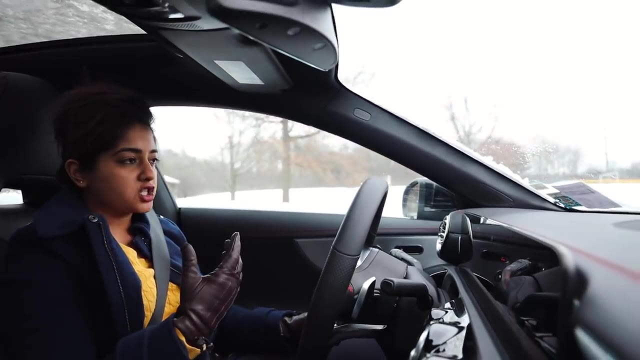 biomedical engineer basically does. My job right now is to work with design development, basically product development of automated molecular diagnostic platforms. I'll take you throughout my day So you'll kind of see a little bit about the work that I do. particularly the area that I specialize in is called lab on chip technology or microfluidics. 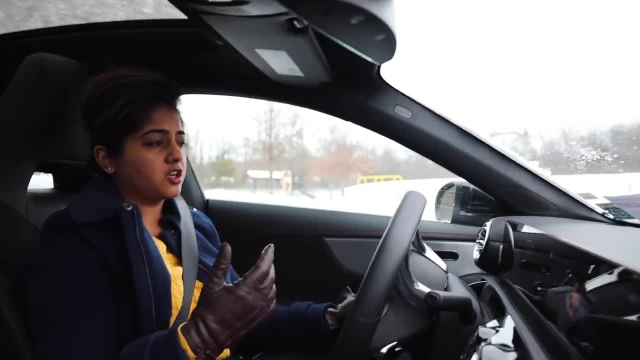 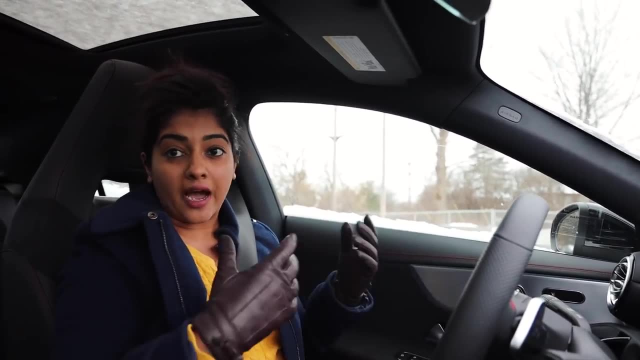 This is basically like: think of every single, like huge lab processes, If we could make a chip out of them. what's the best way to automate these technologies? That's what I work with, So I'm excited I'm going to take you guys along. We are here at work and I'll see you guys in a bit. 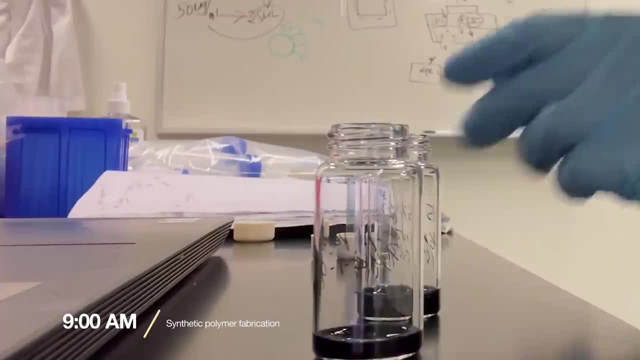 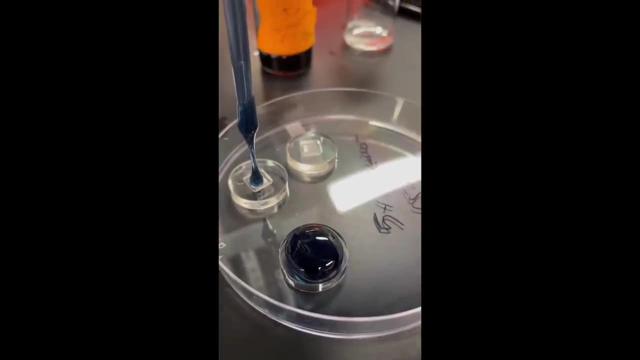 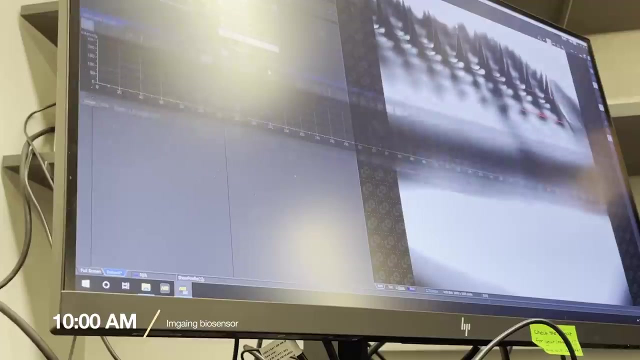 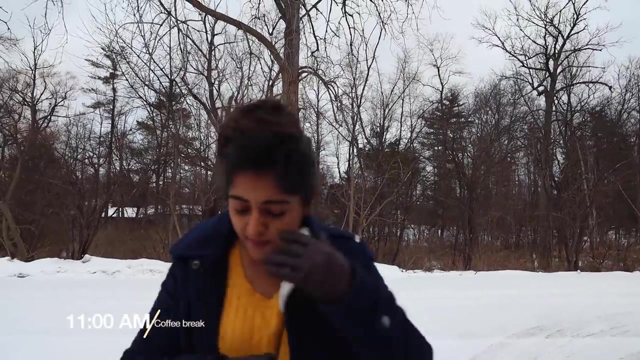 All right, guys. so it's about 11am and it's kind of like my coffee break. So we have multiple buildings I just like to work on And besides, I have a lot of apes to take care of. so I'm just. we have a huge UN metros servicio and also we have some iOS, So a bunch of stuff going on. So 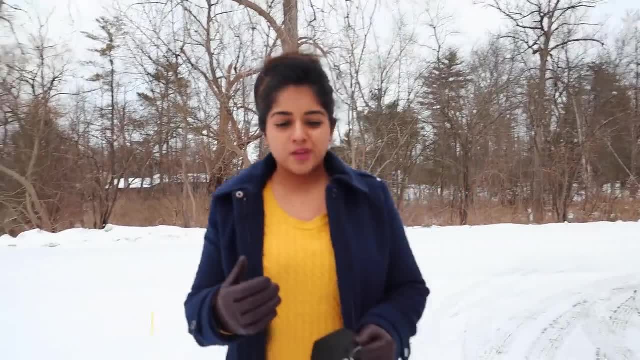 we're going to check out some content over here. I'm going to head over to a cool5.com guys at worked out because he's nice, He at work sometimes. I'm so excited to be here as well. We're going to just go. 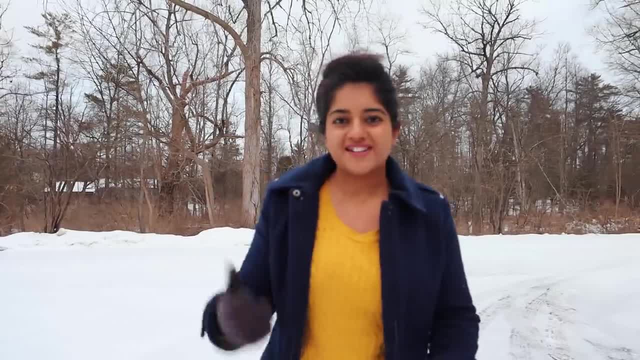 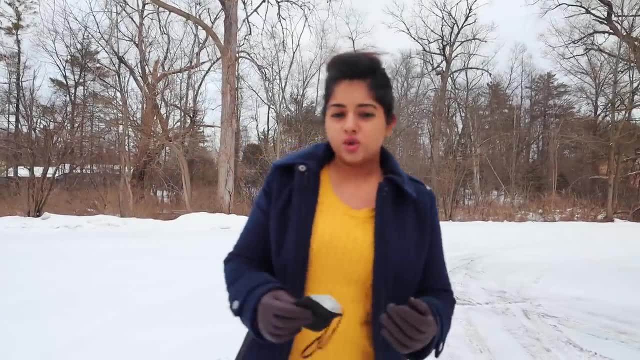 like to walk in between them instead of taking the car, kind of get some fresh air. it's minus 10 degrees today, which isn't really helping, but i thought i would talk to you guys a little bit today and actually tell you what i actually do as a biomedical engineer. so here's the thing. a 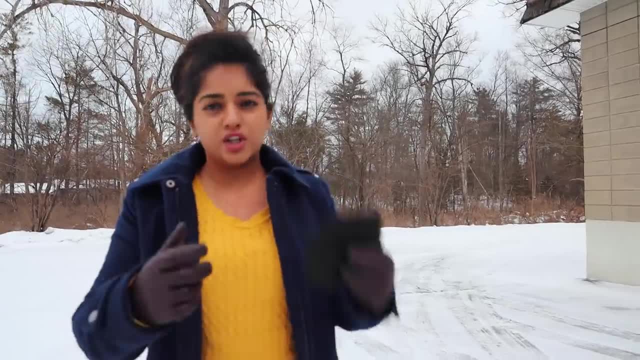 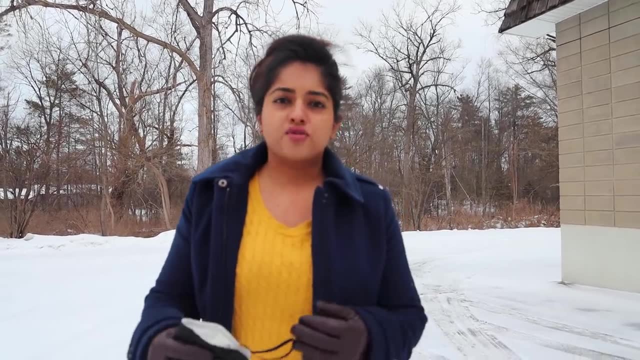 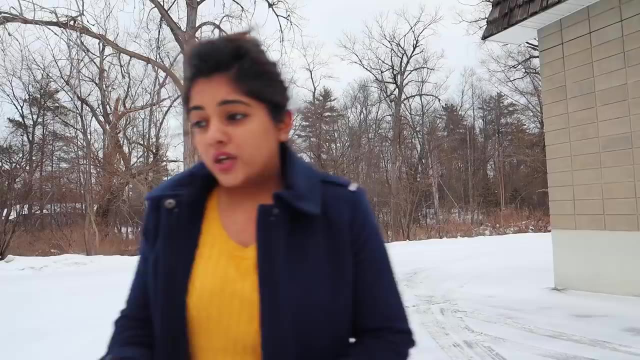 company when it makes like automated molecular diagnostic platforms. there's just so many things involved in that. you know, we do months and months of feasibility testing if we want to introduce a product into the market, and since it's a molecular diagnostic company, we kind of then have to prove out the biology of the entire process, and that's when the bio group comes in. once we have that nailed down and we kind of know that we can reproduce this technology or this product on multiple scales, extensive testing later. that's when engineering and design comes in. where we have, we're given something that works in terms of biology and it's our job to replicate. 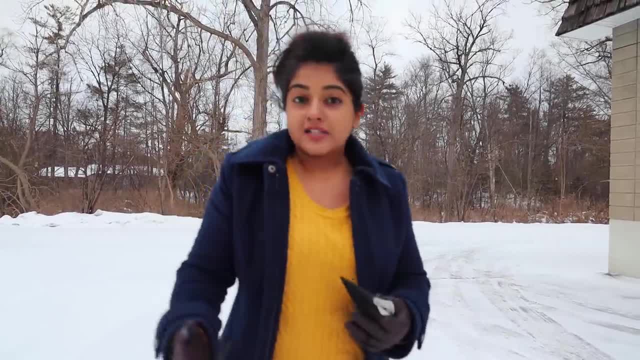 that, and then we're able to introduce it into the market, and we're able to produce it into the market, and we're able to introduce it into the market. and we're able to introduce it into the market that using automation, robotics, liquid handling systems, all that fun stuff. 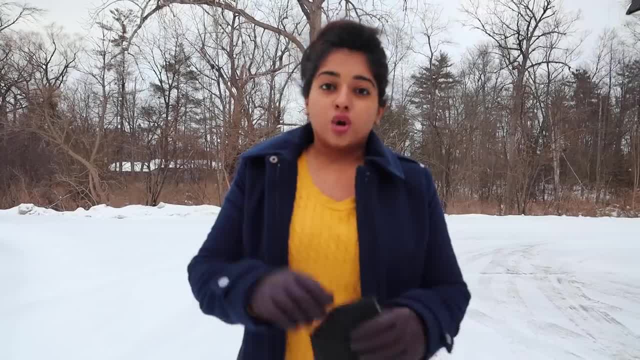 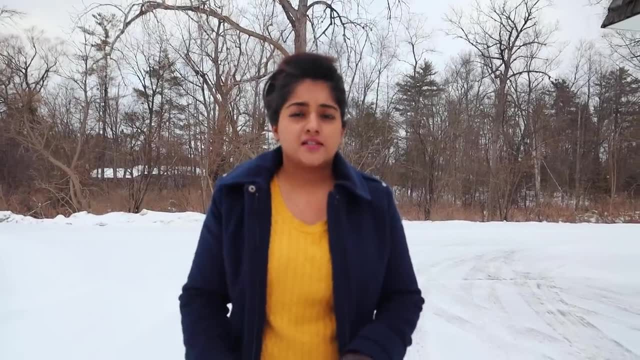 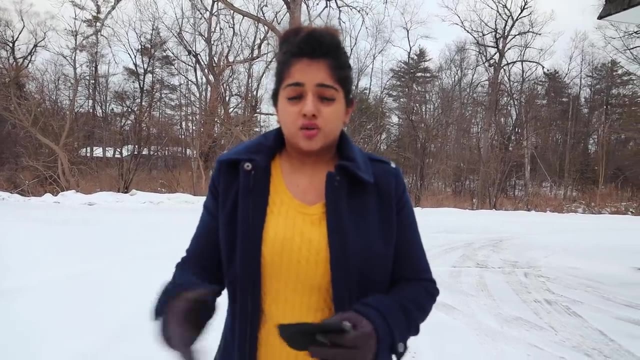 that's basically what my role is, and even after that's all nailed down, when we have manufacturing come in to make these multiple products, there's tons and tons of QC testing because, at the end of the day, we're dealing with biology based products and it's people's lives that these things are testing. so there's a 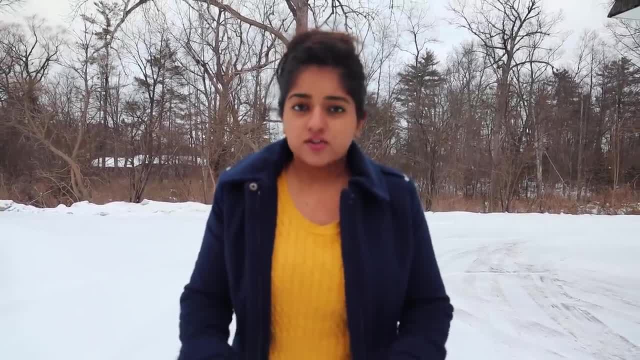 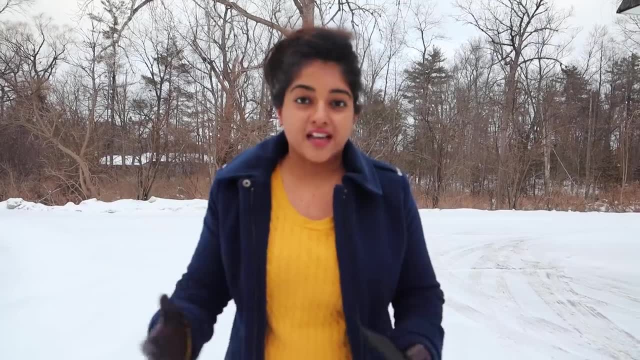 ton of QC testing, FDA rules involved, and all of this is like if one product, a was, was to start from scratch. that's what the product cycle would look like. so that's kind of like the synopsis and the gist of what I do. and in all of this, 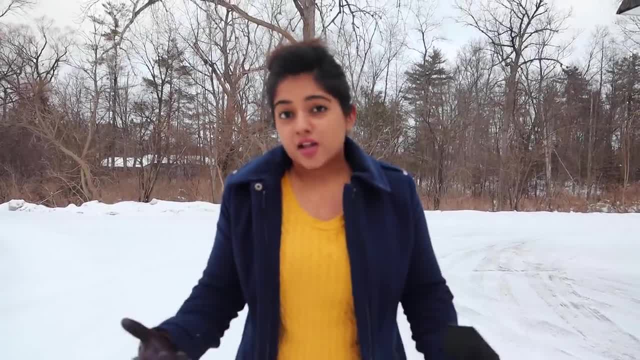 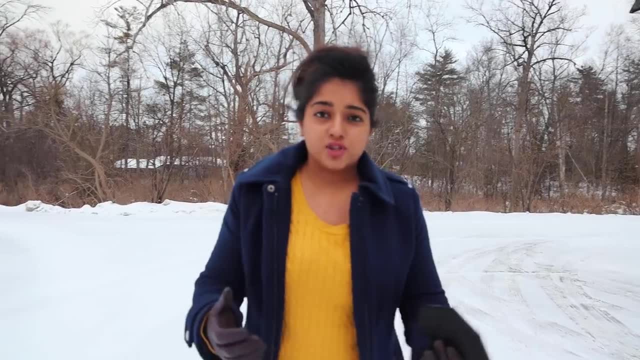 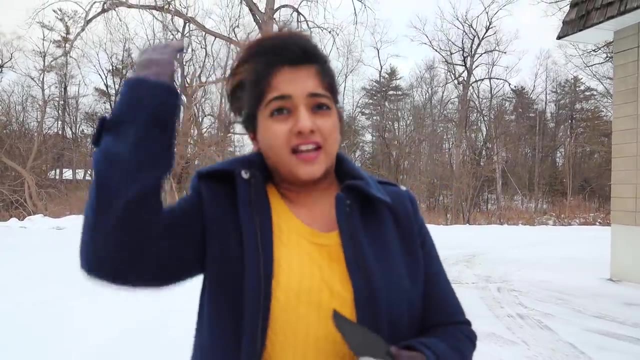 my role is as a design development biomedical engineer and I really have fun at my job. there's a ton of micro fluidics involved, lab on chip, chip technology, which you guys have probably seen a little bit here and there, but I really enjoy it and it's getting really cold here so I'm gonna. 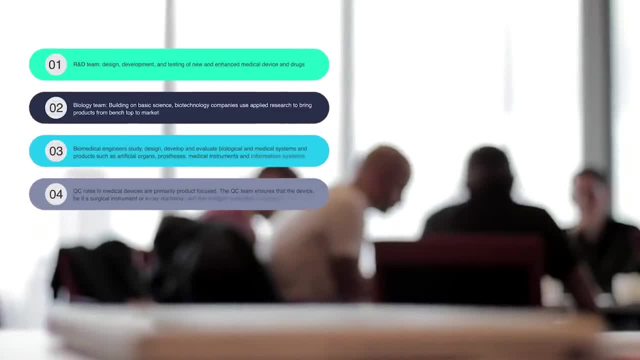 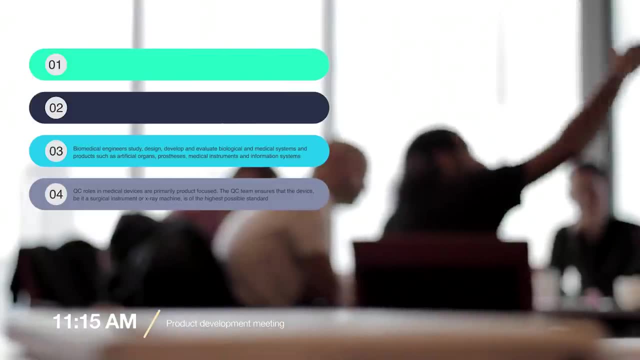 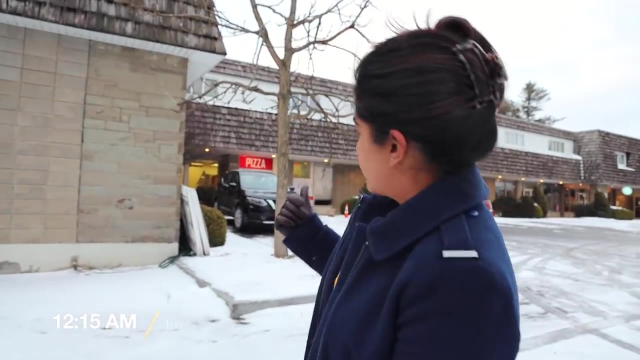 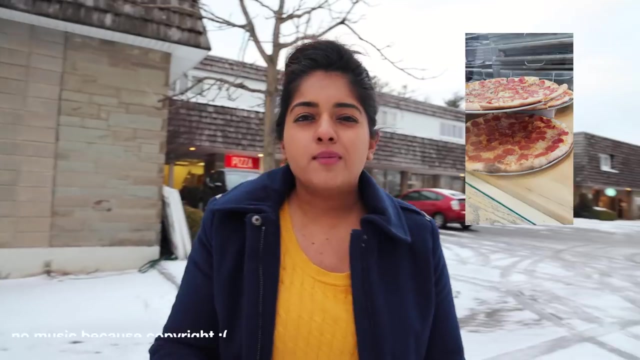 cut this clip. I'll see you guys in a bit. I just wrapped up a couple meetings and came out for lunch. I'm gonna grab some pizza. it's just a neighborhood friendly pizza place. you know. the fun thing is I'll put this on the screen here. a couple days ago I came in in here and I 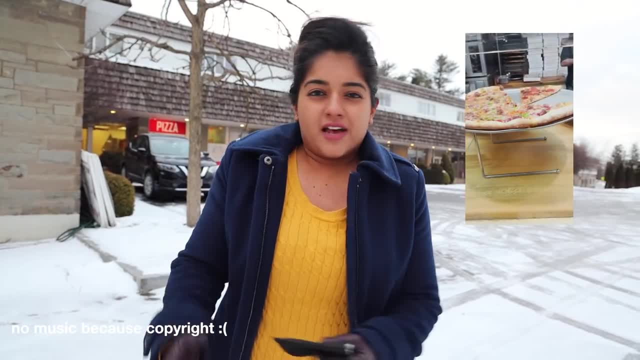 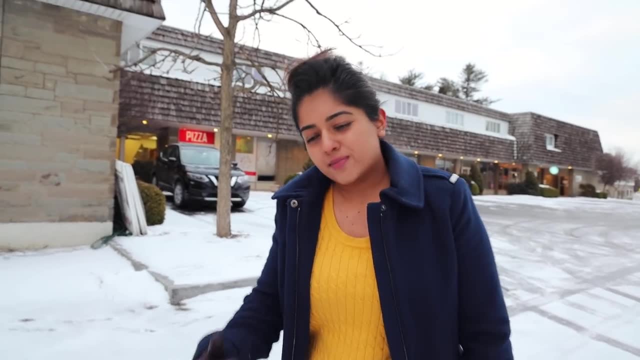 think the people here are like Middle Eastern or something. they were playing full-on punjabi songs and it just made my day. I was just genuinely so happy listening to that. well, we're gonna grab some lunch. I wrapped up a couple meetings in the morning. after this, I have to head to the hospital to get some. 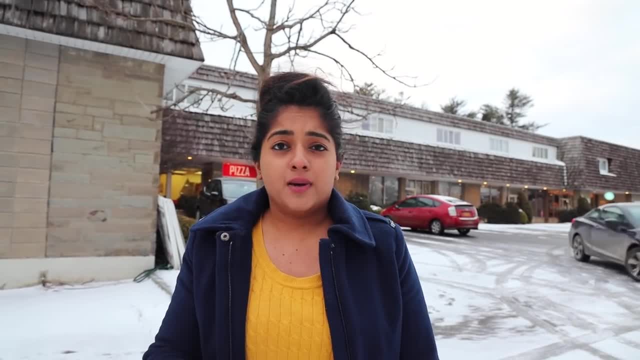 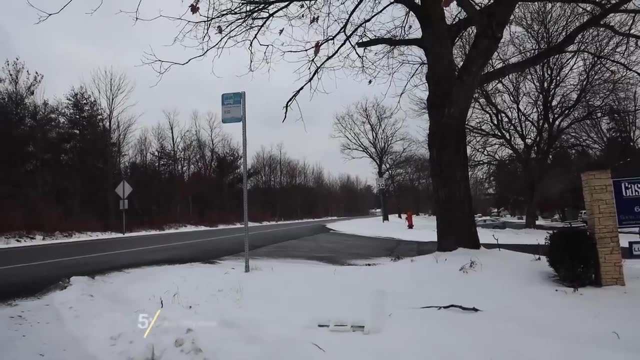 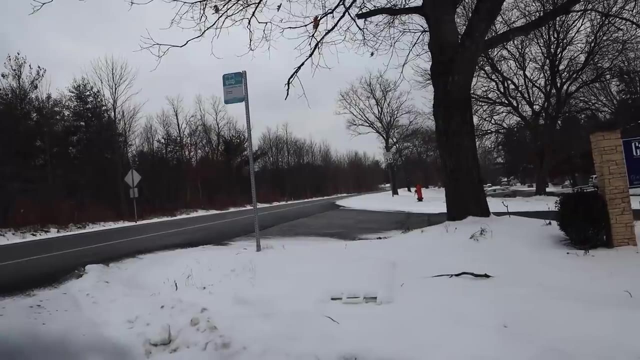 work done, couple trainings, but I'll catch you guys in a bit with more updates. all right, guys. so do you see that that's how the bus stops here are? I know I told you guys that sometimes in the snow it's like covered. There's only some bus stops. Most of them are like that. You just have to wait there for the. 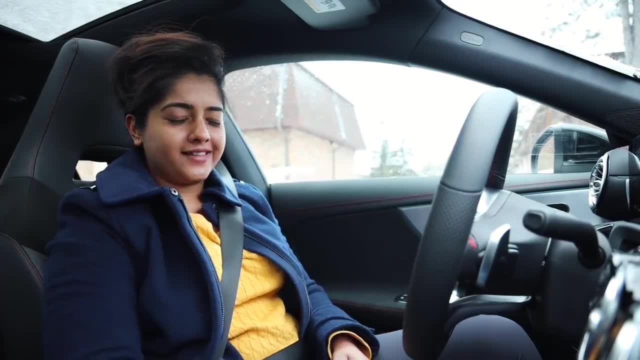 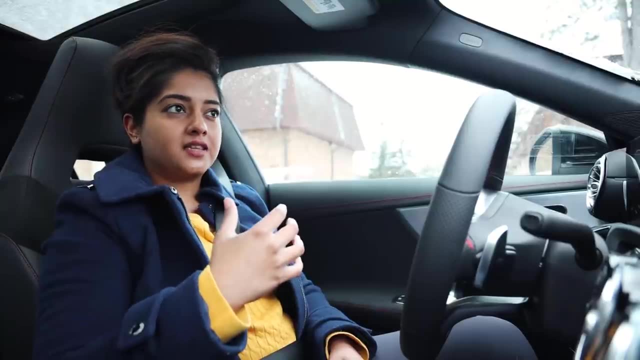 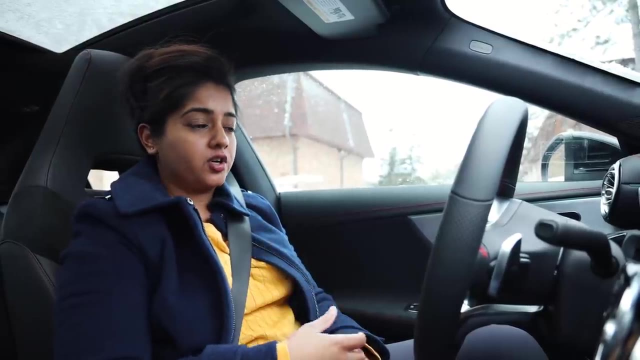 buses to come. So the funny thing is, I started out at that very bus stop. when I came to the US to study I didn't have a car. I came with a mindset that I had to earn my way up, And once I graduated I got a job after maybe a couple months of working. That's when I got my first. 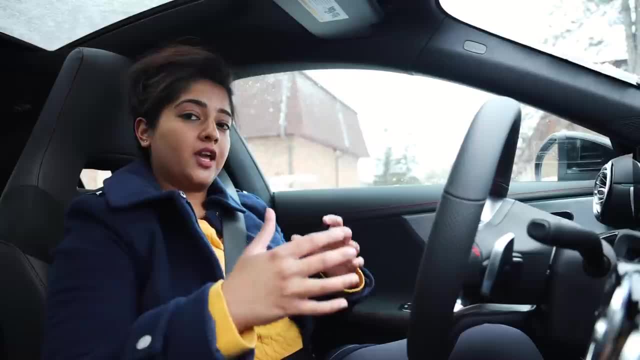 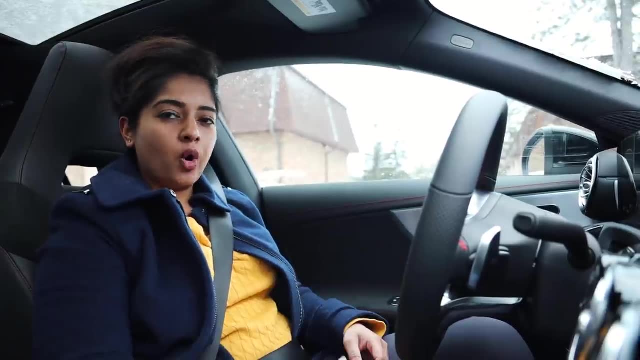 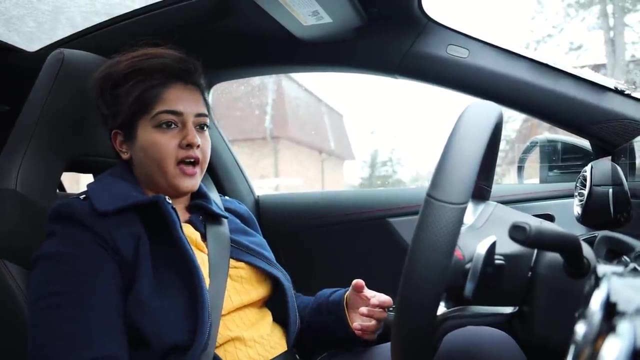 car, which was the Honda Civic, And now I've worked my way up to this Mercedes. I want to make it really clear that it's not at all with YouTube money. My whole aim with the YouTube channel is to give you guys some motivation, inspiration and like a path forward. you know that helps you. 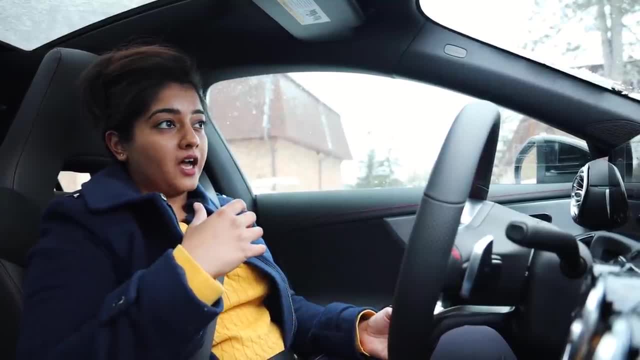 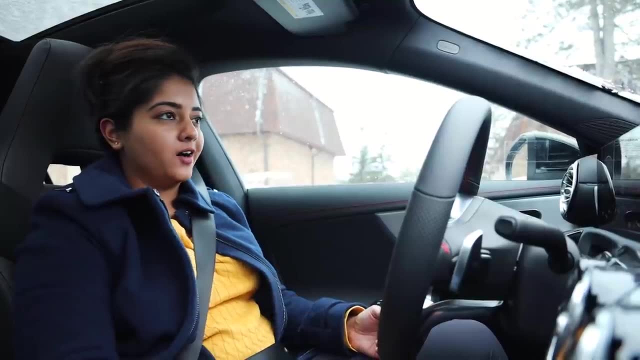 guys, embrace your imperfections. I'm in no way trying to show off with this new car, but I just wanted to address that and get it out there. So you know in all honesty. so it's pretty clear that this car that I've earned, it's through. 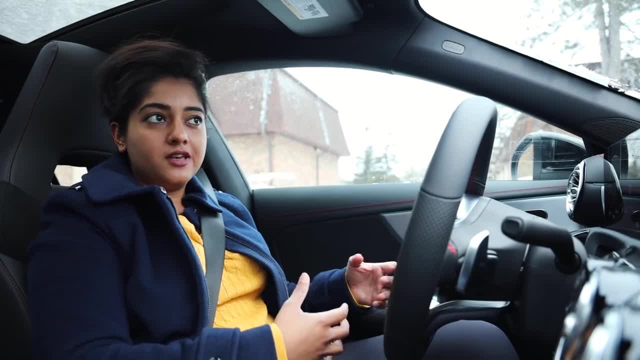 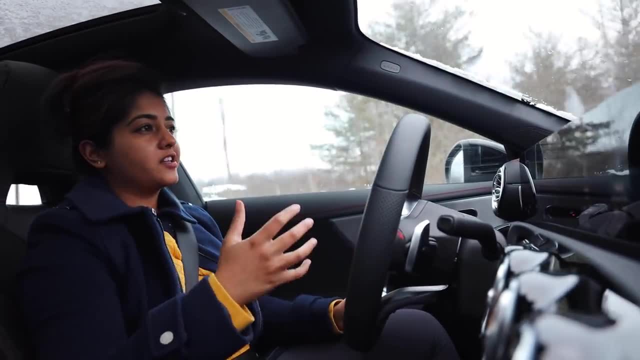 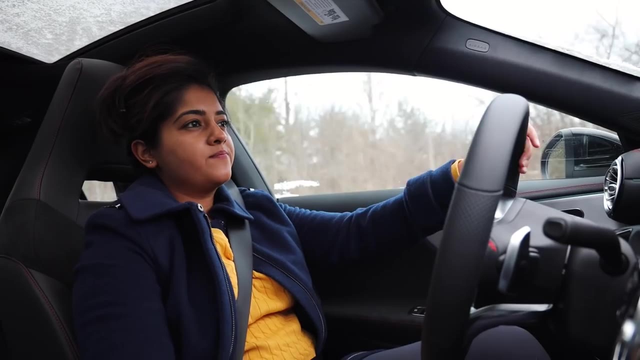 me being a biomedical engineer, not me being crazy Medusa as a YouTuber. So yeah, Right. So it's been a long and tiring day. It hasn't gotten any warmer. The weather is still like minus seven degrees outside and the wind isn't really helping today. But you know, you just have to deal with. 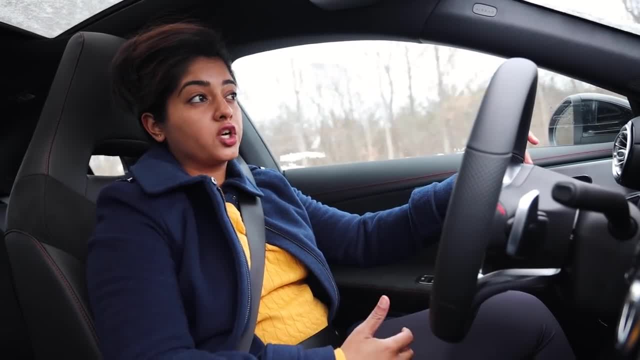 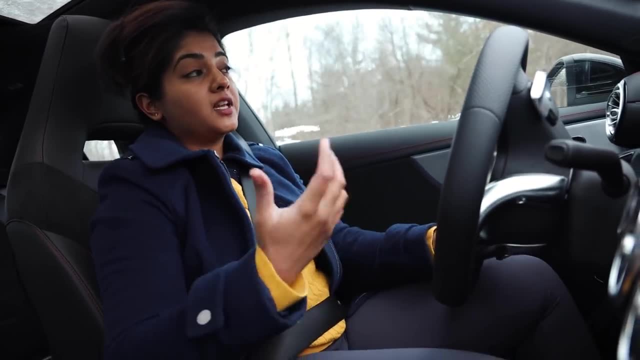 it. Anyways, it's about 5 pm right now. These are usually my work hours. I head to work around eight in the morning and I come back around five. Some days are longer than others, but sometime in between, if I feel like it, I do. 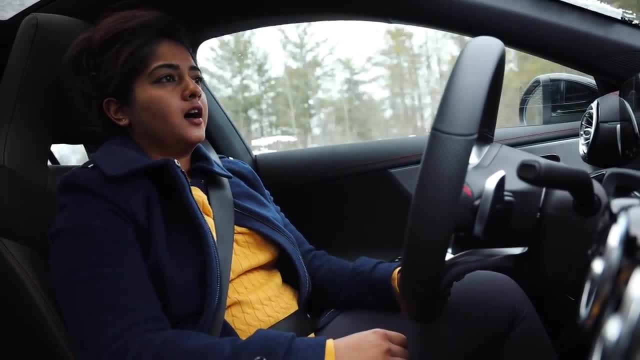 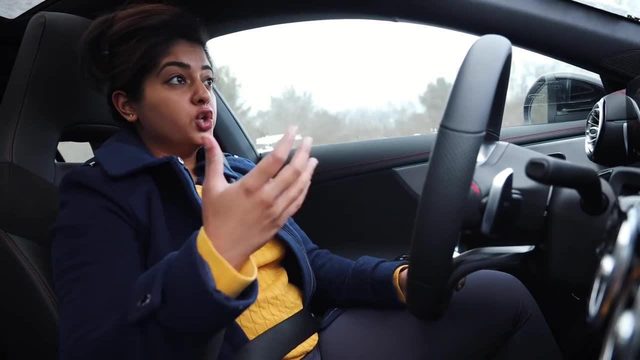 come home for lunch if needed. Otherwise I just eat in the office. But once I go back home, in the weekdays specifically, I have meetings scheduled with a bunch of you guys. It's the mentorship programs. So depending on where students are in the world, 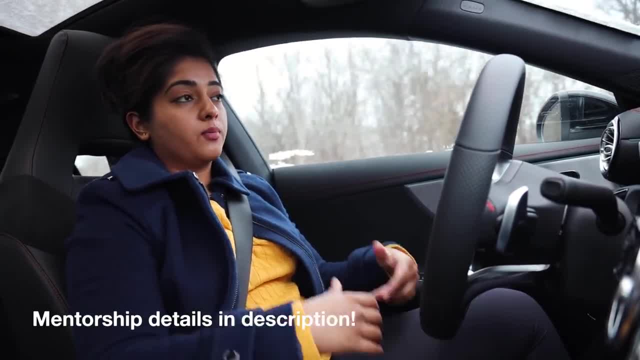 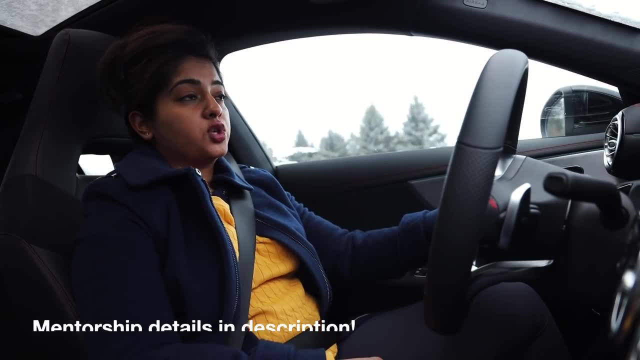 I have meetings with them to make sure they're- you know, making their weekly progress and assure that I'm able to provide the right guidance in terms of whatever help they need. So I have a meeting with one of my students today, So we're going to go home and the meeting 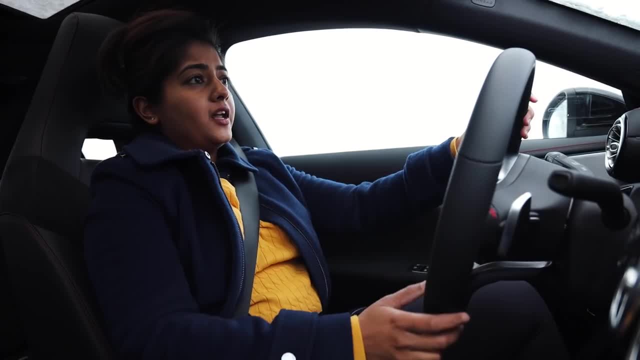 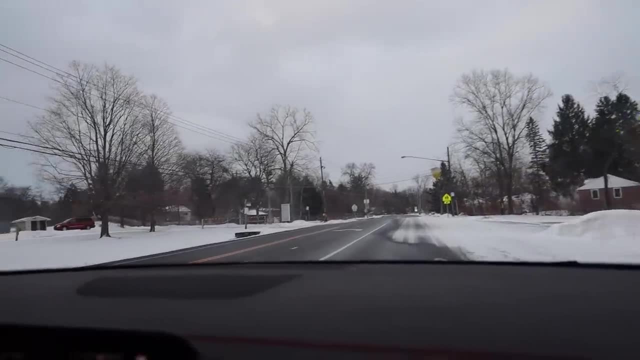 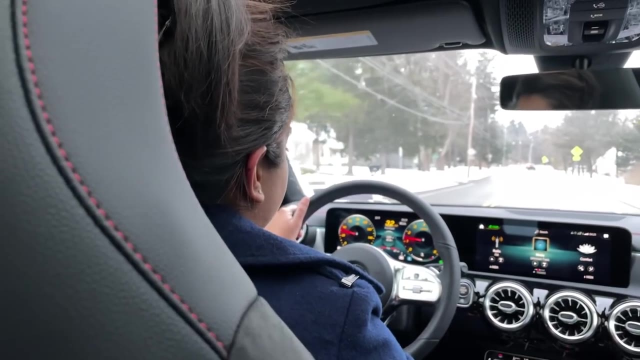 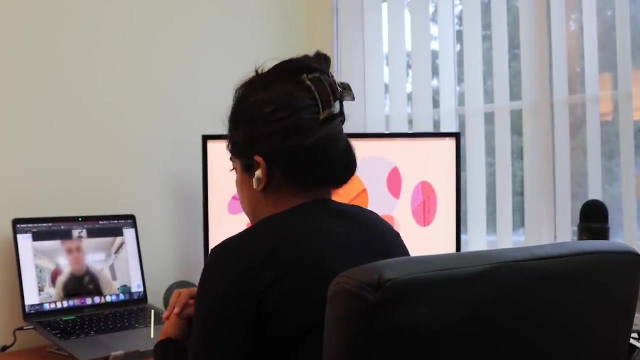 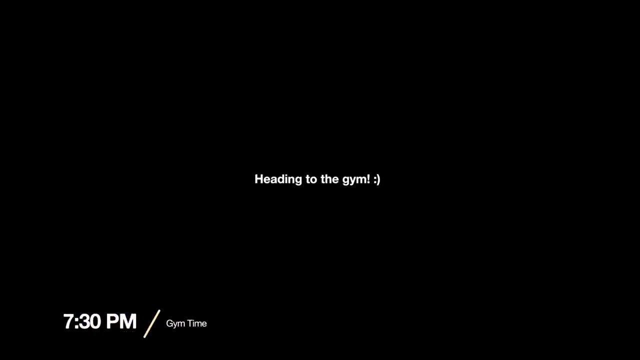 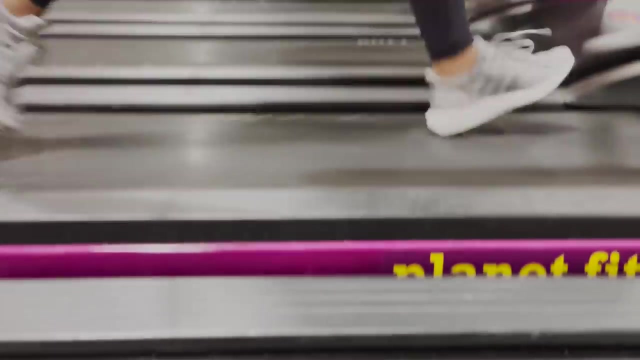 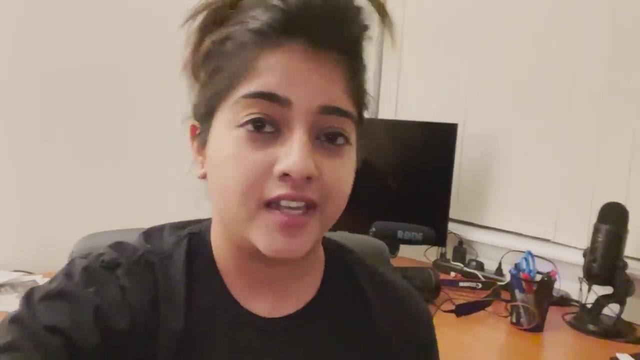 is at 530.. So quickly go change And after that I'll catch you guys in a bit. All right guys, it is 11 pm And I am pretty much exhausted. I just got home from the gym. This is pretty much how every day. 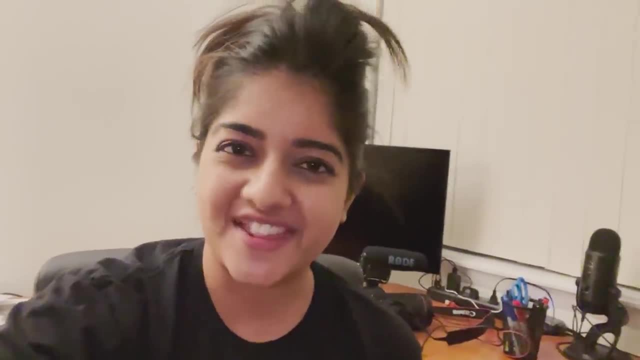 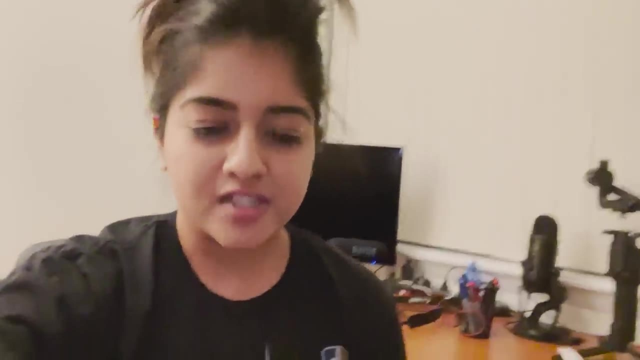 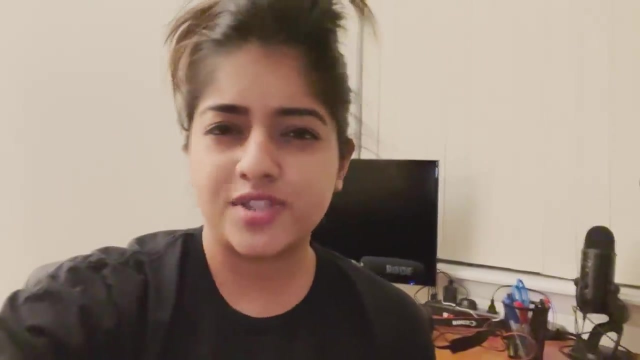 is here and there, Find some time to do basically everything, But I think like the one thing that I can't survive with is just skipping the gym. For me, going to the gym is like something that relieves my stress. I feel really, really productive after I get a good workout. So do you guys have something? 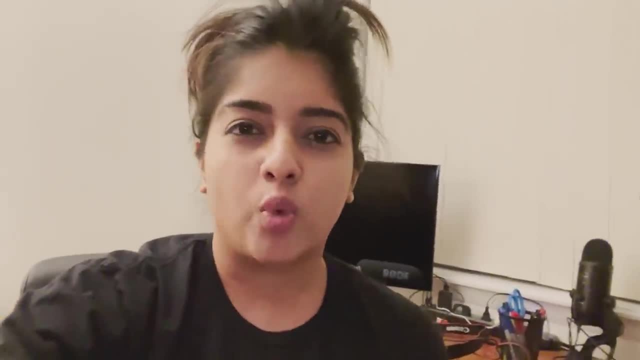 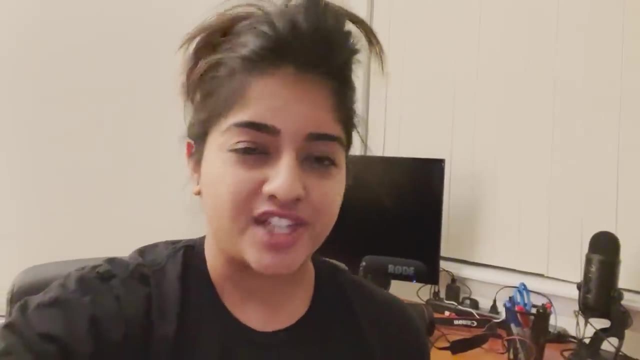 like that. I mean comment that down below. That's today's question. What's the one thing that you would never skip? How busy or tired you are in a day- Hashtag: crazy Medusa, And I'm going to wrap up the video, right.